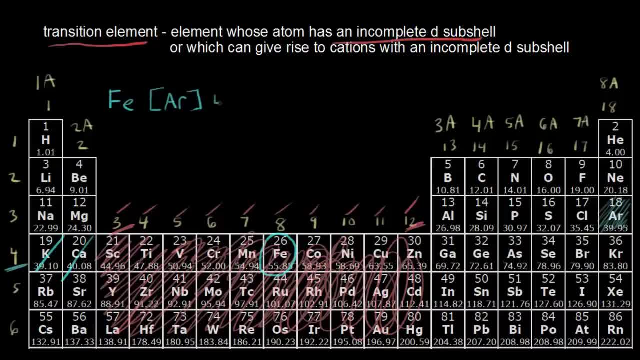 I can say that would be 4s1,, 4s2, so I can write 4s2 here. Then I'm in my D orbitals Again, just looking at the periodic table to write my electron configuration, I would say one, two, three, four, five, six electrons. 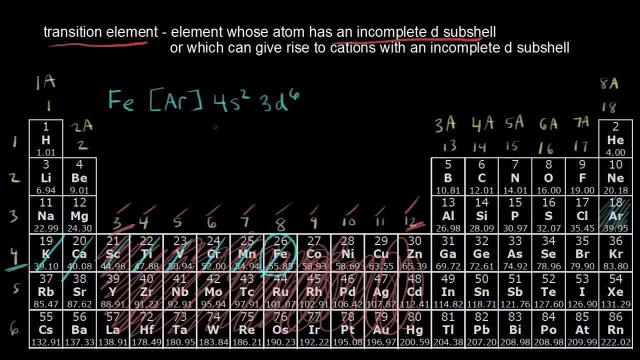 That would be 3d6.. I could have written this: 3d6, 4s2.. Right now, both are considered to be correct answers. I won't get into a discussion about the order of filling of these orbitals in this video. 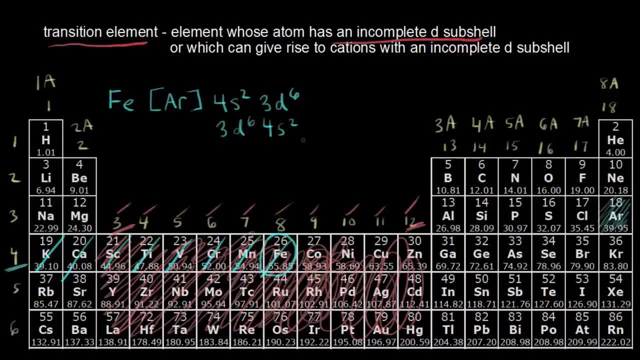 so I'll save that for another video. This video is only talking about definitions and identifying elements on the periodic table. Either one of these would be a correct electron configuration. When I look at the D orbitals for the electron configuration, I can see that there are six electrons in my D orbitals. 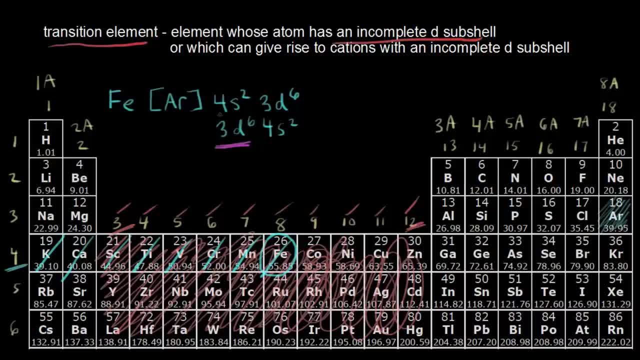 That's an incomplete D subshell, because I can fit a total of 10 into my D orbitals. Iron would be an example of an element whose atom has an incomplete D subshell. Iron is a transition metal. Let's write the electron configuration for zinc. 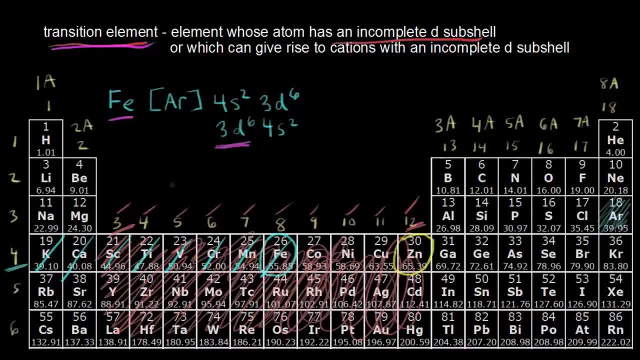 Let's find zinc over here, right there on our periodic table. I wanted to write the electron configuration for zinc. Once again, I would go to the noble gas before it, which is argon. I would put in brackets argon right here. 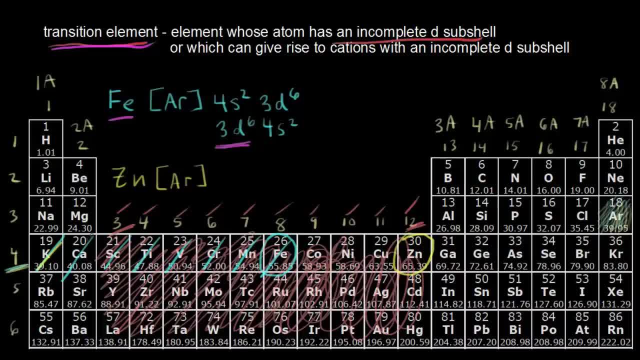 Once again it takes me to the fourth energy level, 4s1,, 4s2.. Then I count over for my D electrons: 1,, 2,, 3,, 4,, 5,, 6,, 7,, 8,, 9, and 10.. 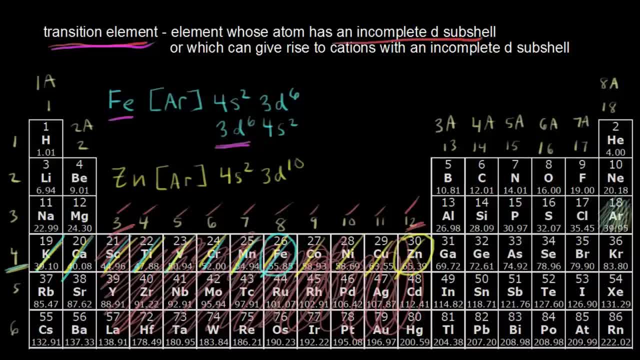 It would be 3d10.. Once again, I could have written that argon in brackets 3d10, 4s2.. It doesn't matter. Let's think about the definition for a transition metal, an element whose atom has an incomplete D subshell. 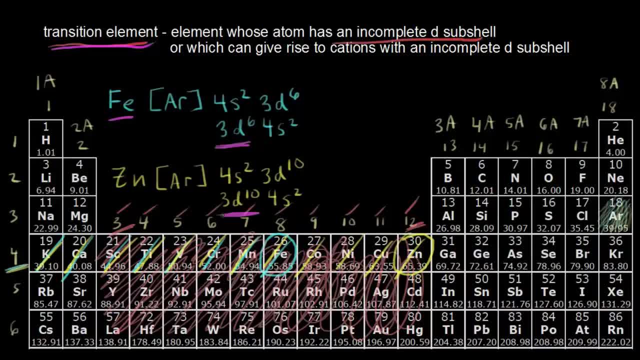 If I look at the D orbitals for zinc, they are completely full. I have 10 electrons in my D orbitals. This is a complete D subshell. This does not meet the definition for a transition element. Also in the definition it talks about cations. 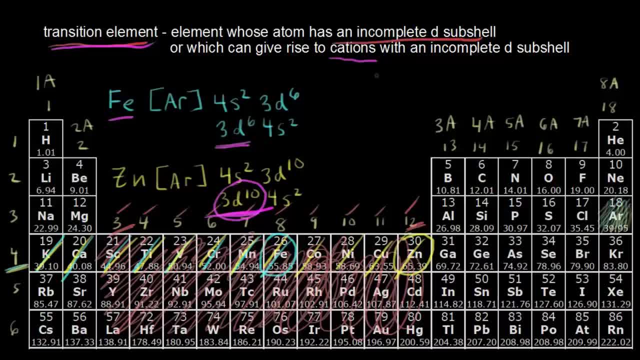 Let's think about the cation that zinc would form. Zinc would go to zinc 2+. If I wanted to write the electron configuration for zinc 2+, I need to think about where does zinc lose two electrons If you're going from a neutral atom of zinc? 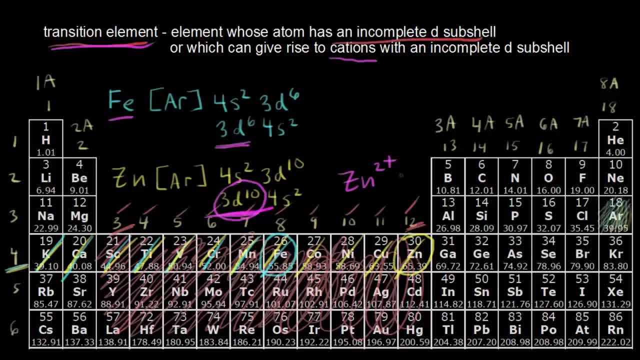 to zinc 2+, you would have to lose two electrons. I already know that those two electrons are going to be lost from the 4s orbitals. We're going to lose these two electrons right here on your electron configuration. You'd be left with 3d10. 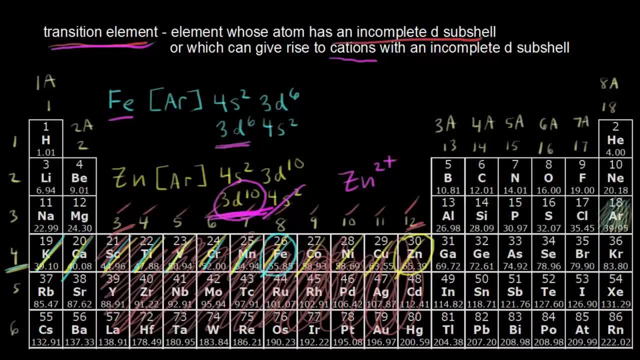 Once again, you have a cation that has a complete D subshell. You've completely filled your D orbitals. The cation does not have an incomplete D subshell, which means that it doesn't fit our technical definition for a transition element from IUPACs. 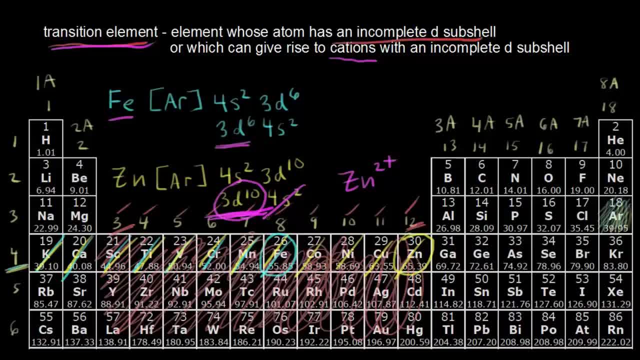 Once again, there are two ways of thinking about it. One is a very general way. You might hear someone talk about an element from groups 3 to 12 as being a transition metal, Or you might find people who are a little bit more particular about the definition. 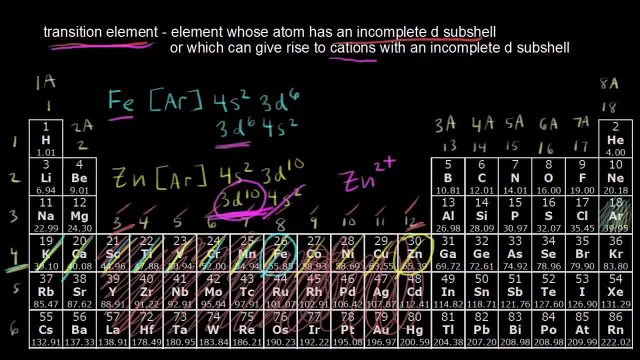 who go along with IUPAC. It's good to be aware of both ways of thinking about it.